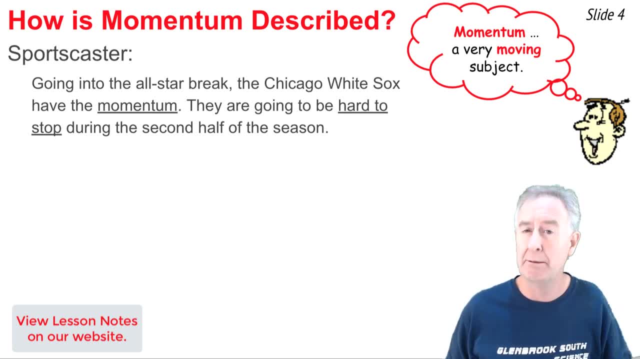 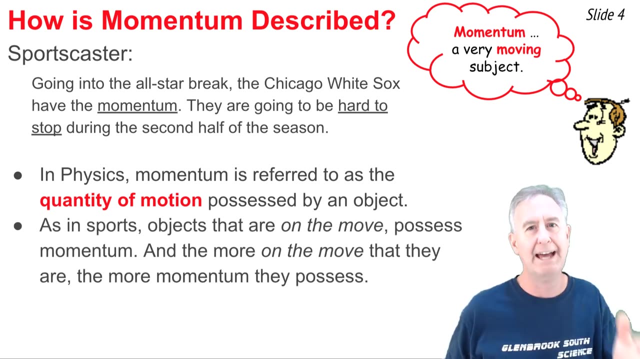 Well, they may not say that. They may not say that about the Chicago White Sox, but they probably say it about your favorite sports team. The fact is that momentum is a physics concept And in physics, momentum describes the quantity of motion that an object possesses. And, just like in sports, an object that is on the move has momentum, And the more on the move that it is, the more momentum that it possesses. And, just like your favorite sports team, objects that have momentum are going to be difficult to stop. 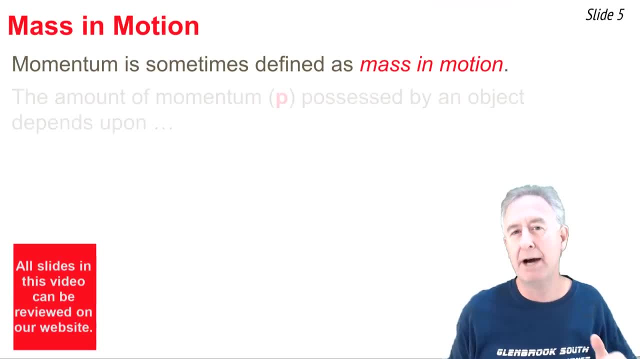 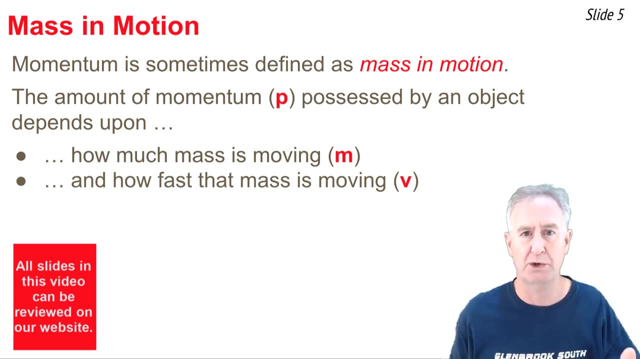 Momentum is sometimes called momentum. Momentum is sometimes defined as mass in motion, And the amount of momentum an object possesses depends upon two variables: how much mass is in motion and how fast that mass is in motion. Now, when we write a formula, it has to express these two dependencies between momentum and the two variables that affect it. And we'll write that formula using symbols. 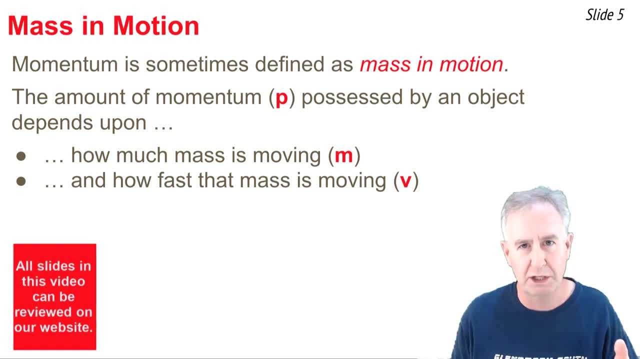 Now the symbol for mass is the symbol m, as it has always been, And the symbol for velocity is the symbol v, as it has always been. Velocity describes how fast an object moves And in what direction. More on that later. 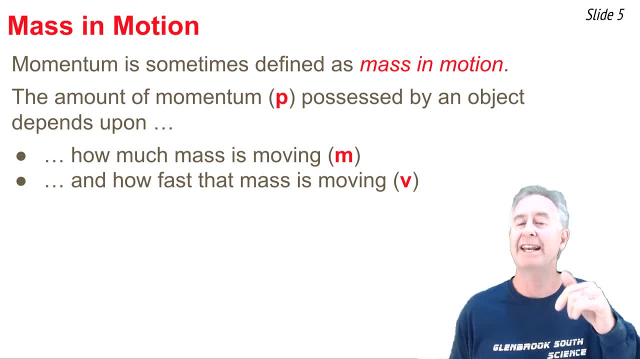 So when we write the formula, we're going to have to use something other than m for momentum, And the symbol that has traditionally been used is the symbol p for momentum. So this formula is going to have to express the idea that momentum depends on mass and velocity. 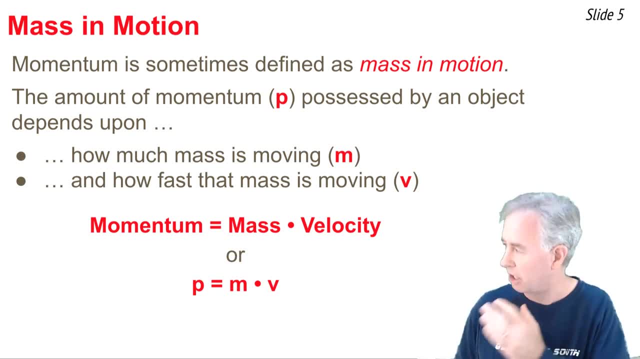 And it looks like this: Momentum equals mass times velocity. Or, putting symbol form, p for momentum equals m for mass, Multiplied by v for velocity. Now, whenever we get a new formula or a new quantity in physics, it's common to use the formula for it in order to define the units typically used to express the amount of momentum. 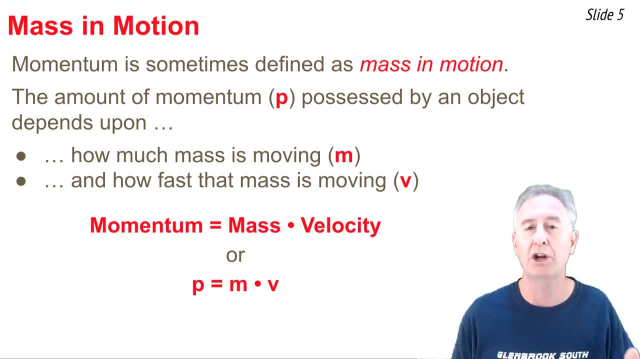 So, based on this formula, we would reason that the units of momentum are units of mass multiplied by units of velocity. The standard metric units would be a kilogram times a meter per second. Other units would have to express the same equivalency between momentum and mass. 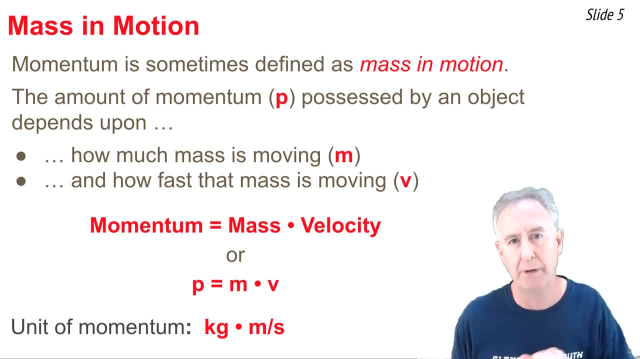 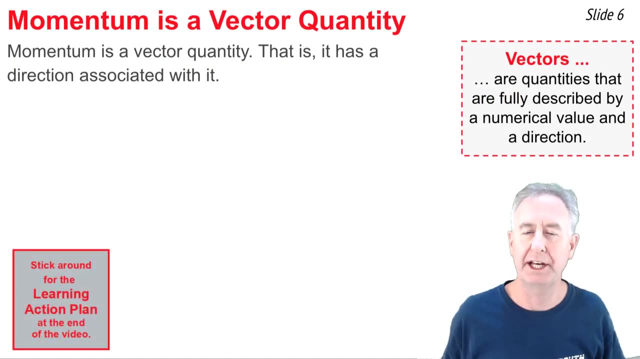 And be a mass unit multiplied by a velocity unit, Like a kilogram times a kilometer per hour Or a gram times a centimeter per second, But the standard metric unit is kilograms times meter per second. Momentum is a vector quantity And in describing it as a vector quantity, what we mean is it's not fully described until you've included both a magnitude and a direction. 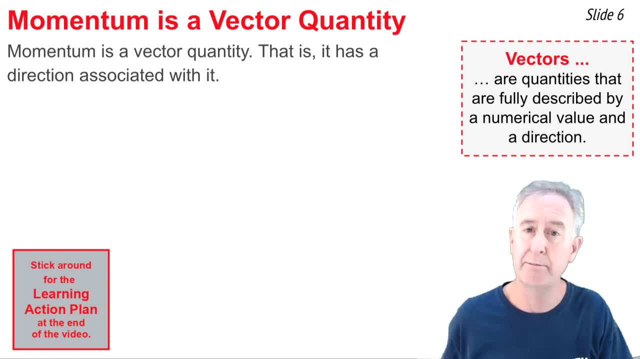 Now, by magnitude we mean numerical value or number, And by direction we mean North or South, And by direction we mean North or South, East or West, Right, left, etc. So in order to fully describe momentum, we need to have a rule for describing the direction of the momentum. 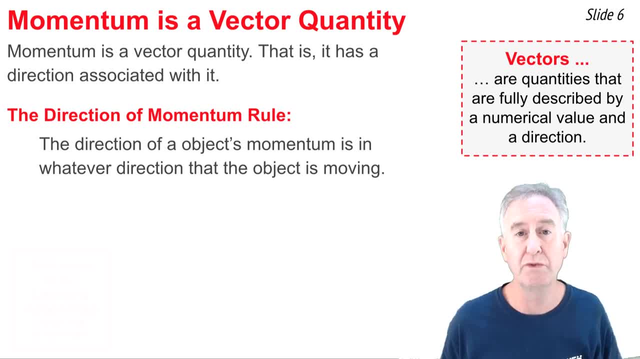 And the rule is really very simple. It's whatever direction an object is moving. that's the direction of the momentum. So what that means is that if an object is moving east, it has an eastward momentum, And if an object is moving down, it has a downward momentum. 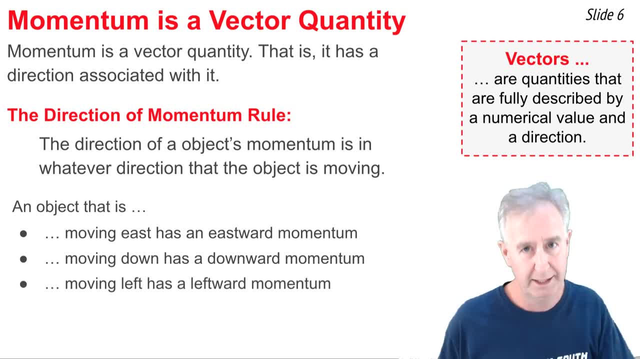 And if an object is moving left, it has a leftward momentum. That's pretty simple, Unless you become distracted by external factors Or extraneous information, like an object speeding up or slowing down. So just to make sure you got it, if an object is moving left and slowing down, it doesn't matter. 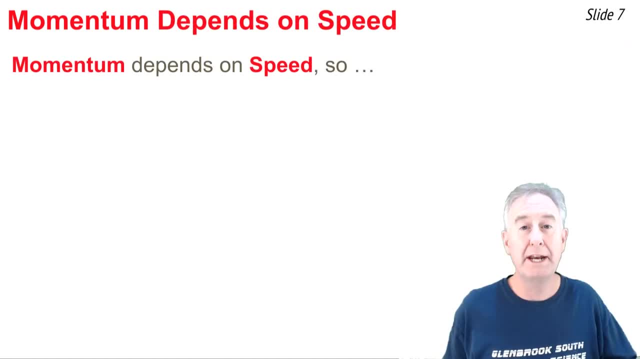 It still has a leftward momentum. Now, momentum depends upon speed, So you could reason that what is ever happening to the speed during any period of time is also happening to the momentum. For instance, if an object is increasing its speed, it's increasing its momentum. 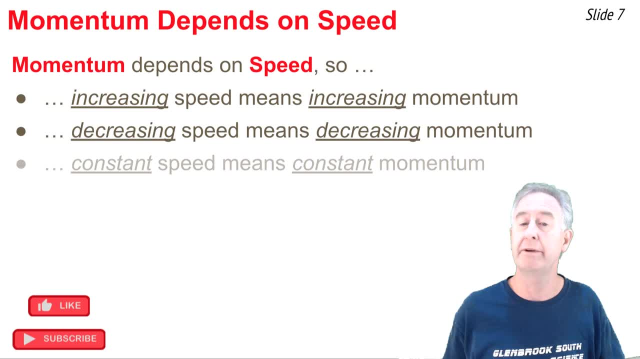 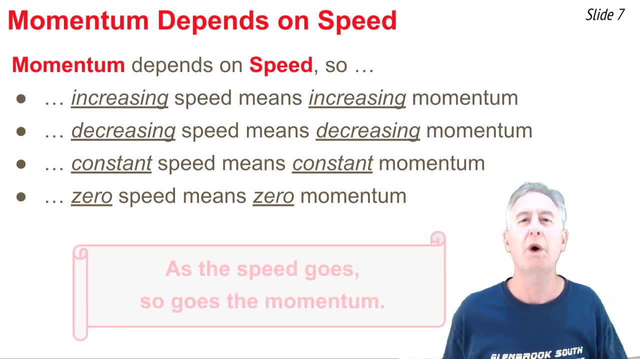 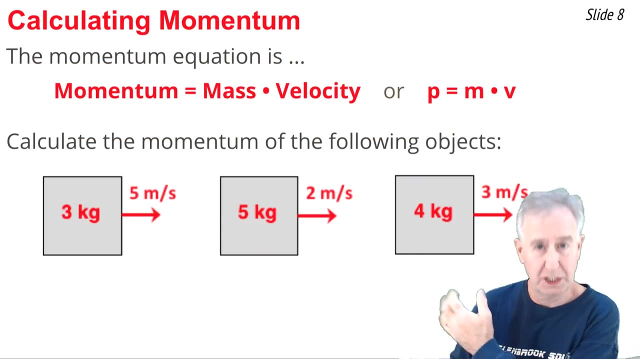 If it's decreasing its speed, it's decreasing its momentum. If it has a constant speed, it has a constant momentum, And if it has zero speed, it has a zero momentum. However, the speed goes, so goes the momentum. When you have to calculate the momentum, you of course need to use the formula. 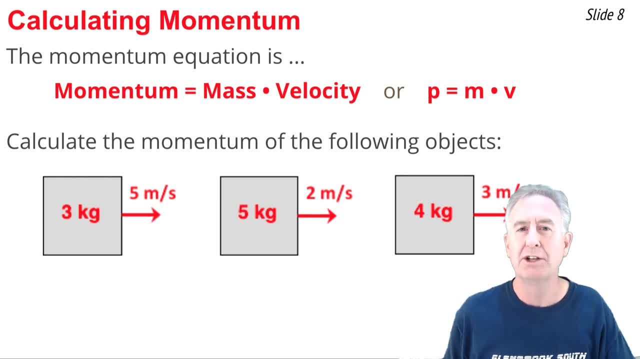 P momentum equals m times v. So you look for the mass, you look for the velocity and you multiply. So here's three quick examples. In the first example the mass is 5, and the velocity is 3.. 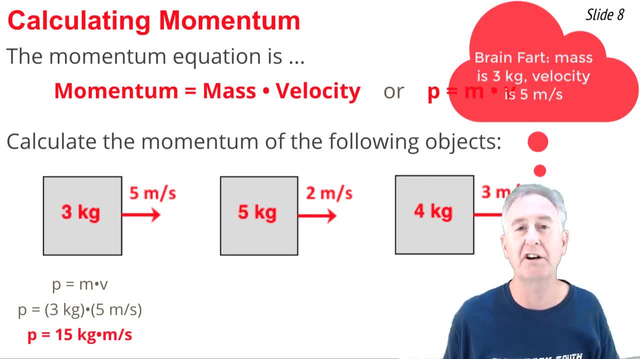 So you multiply and you get 15.. And the units are kilograms times v. In the second example the mass is 5, and the velocity is 2.. So when you multiply you get 10 kilograms times meter per second. 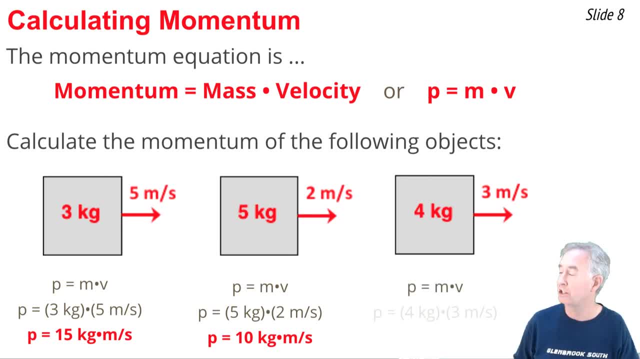 And in this last example the mass is 4, and the velocity is 3.. So you multiply and you get 12 kilograms times meter per second. Now this was quite easy, but if you had more difficult numbers you'd still do the same thing. 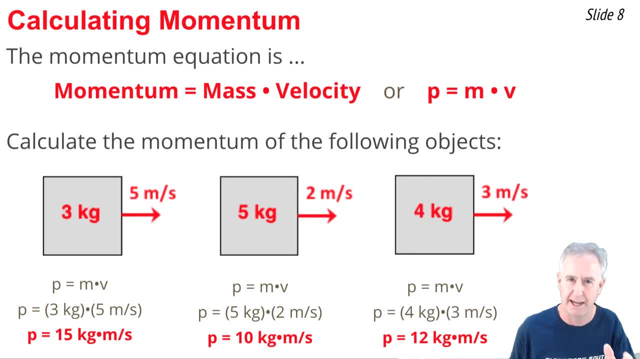 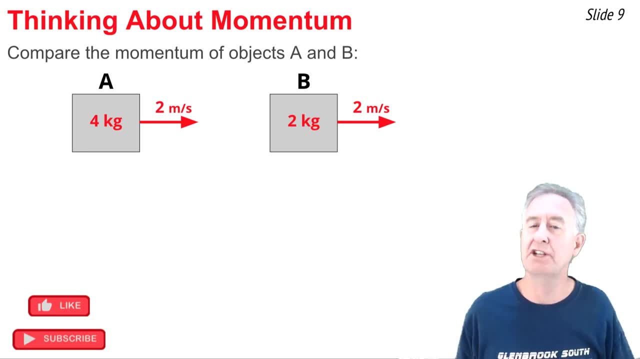 Make it easy, maybe pull out your calculator and multiply mass times velocity. In the previous three calculations we used a formula- P equals m times v as a recipe for calculating some numbers. Now we're going to use that formula differently. 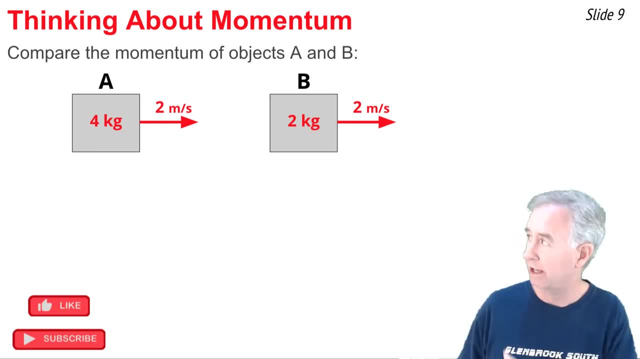 As a guide to thinking about how to compare the momentum of two objects like objects A and objects B. When you look at the diagram you notice they have the same velocity But object A has twice the mass. So using the formula, we would reason that the momentum of object A is twice the momentum of object B. 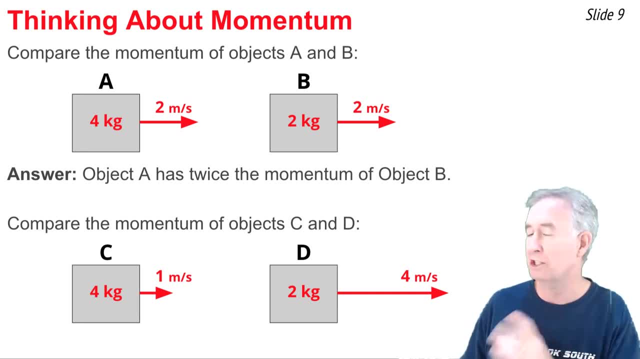 Our second example is a little bit more difficult, because we have objects C and D, and D has one half the velocity as object C, But D also has four times the speed of object C. So we would reason that with half the mass but four times the speed. 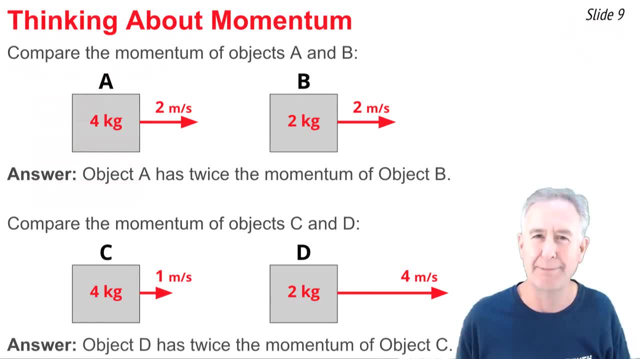 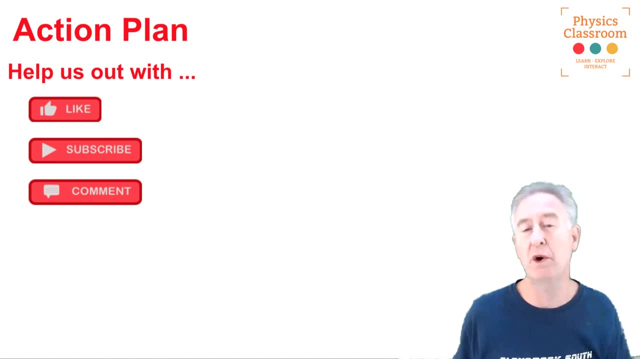 that object D has twice the momentum of object C. And now I'd like to leave you with an action plan, a series of next steps for making the learning stick. Before I help you out with that, could you help us out? If you like the video, give us a thumbs up. 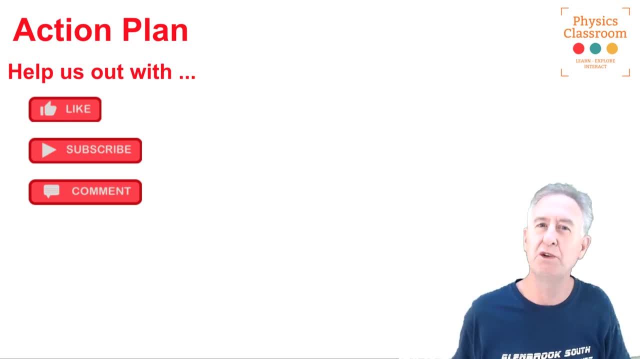 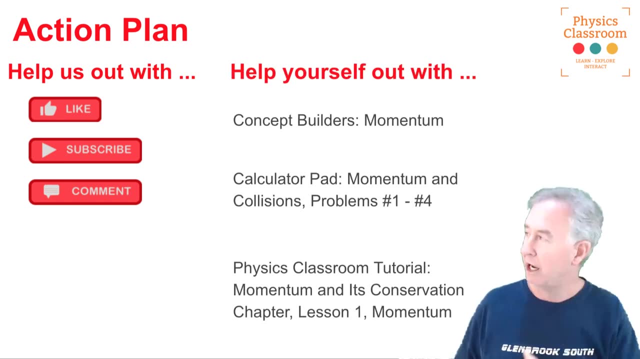 Subscribe to the channel, Tap on the bell to get notifications when new videos come out, Or simply leave a question or comment in the comment section below. Here's your action plan. Here's three items from our website, the links to which are in the description section below. 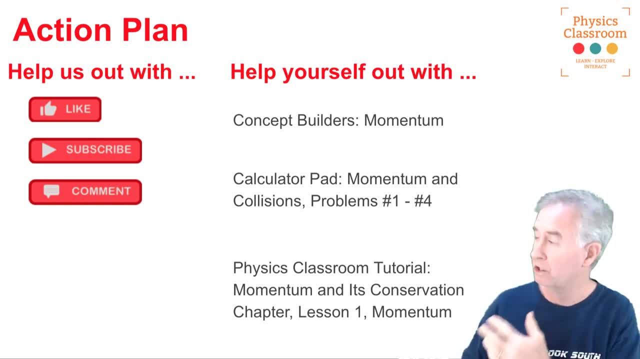 Any one of which would really help solidify your learning. The first is a concept builder, A great practice for the conceptual ideas in this video. Then there's the calculator pad if you need help with calculations. You'll get questions, you'll get answers and you'll get audio-guided solutions. 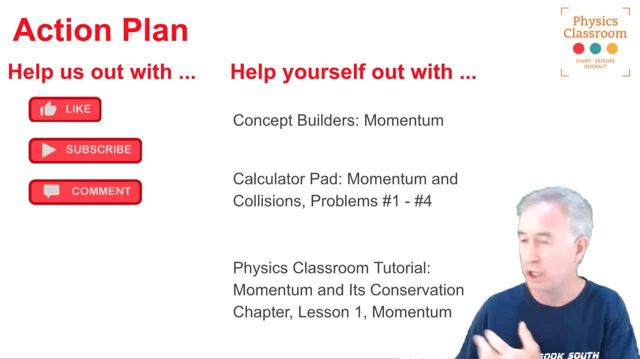 And finally, if you need a reference or something to read, check out our tutorial section, An easy to read physics tutorial that will help you out with any concept. You'll find links to every one of these in the description section below. Whatever you do, I wish you the best of luck. I'm Mr H and thanks for watching.